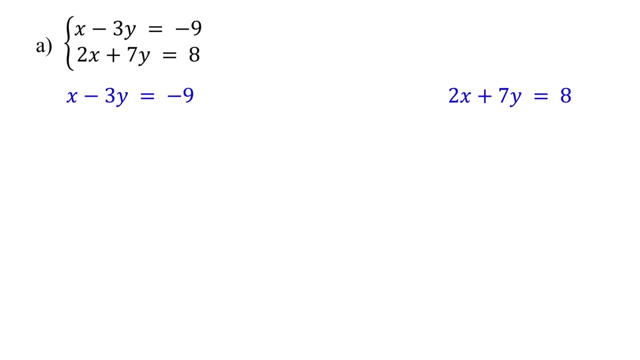 making it easier to isolate x in the first equation. So let's go ahead and do that. Add 3y to both sides of the equation. These cancel out and you get x equals negative 9 plus 3y. Now that we have x by itself, the next step is to substitute this expression. 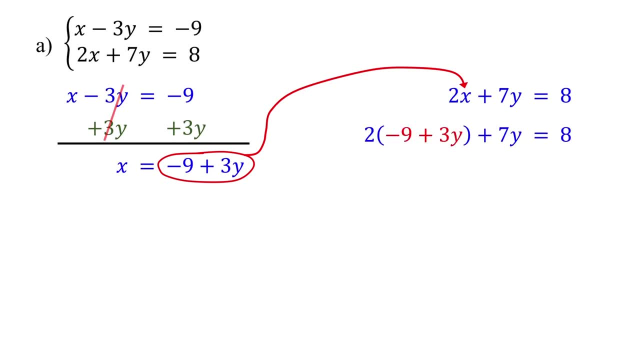 with the equation of x Into the second equation for x. That is why it is called the substitution method. As you can see, we now have an equation with just one variable, and we know how to solve this right. First, let's distribute the two. 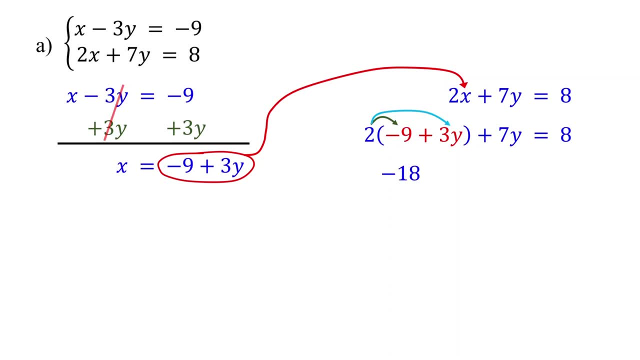 2 times negative. 9 is negative 18.. 2 multiplied by 3y equals 6y. Then combine like terms: 6y plus 7y equals 13y. Then add 18 to both sides of the equation. On the left side the 18s cancel each other out. 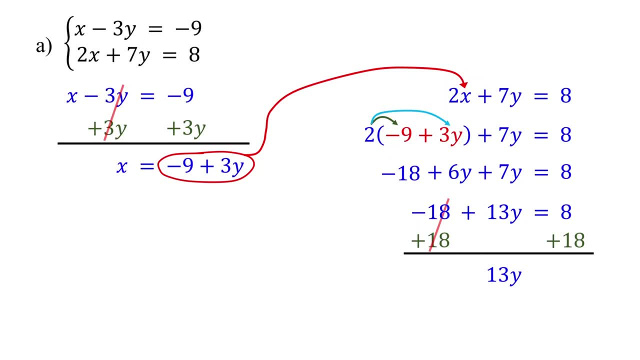 leaving us with 13y On the right side. 8 plus 18 is 26.. Now to isolate y, divide both sides by 13, and you get y equals 2.. Now that we have the value of y, the next step is to find the value of x. 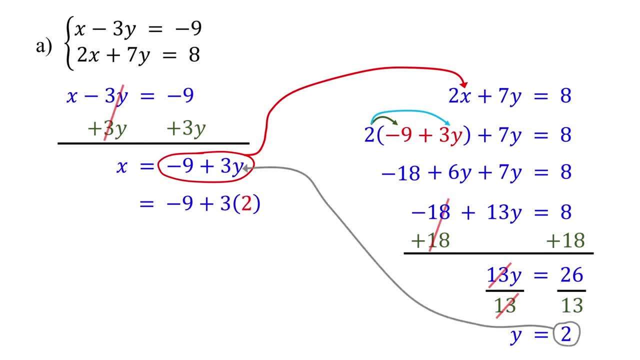 by plugging in 2 for y. in this equation, which is basically the first equation solved for x, 3 times 2 is 6, and negative 9 is negative 9.. 9 plus 6 is equal to negative 3.. Finally, write your solution as an ordered pair. 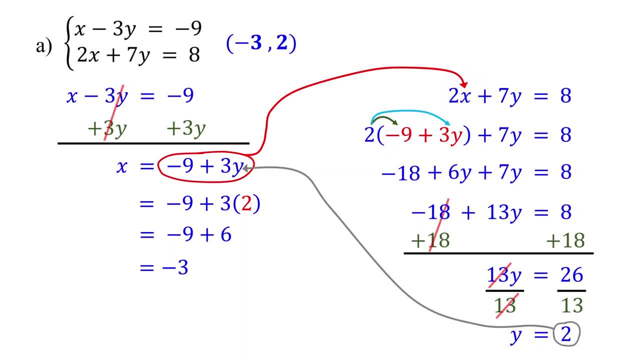 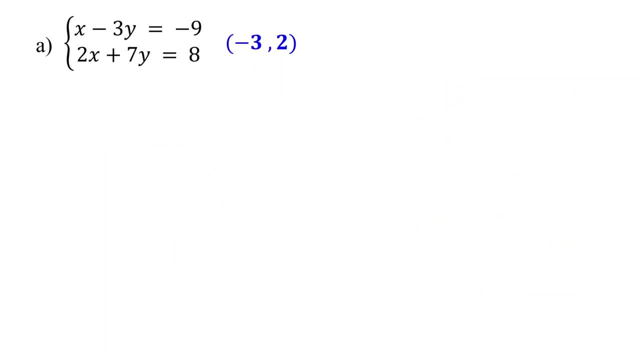 negative 3 comma 2, with x equal to negative 3 and y equal to 2.. If you were to plot the graphs of these two equations, the lines would intersect at a point. negative 3 comma 2.. We can check that the ordered pair is a solution to the system by substituting: 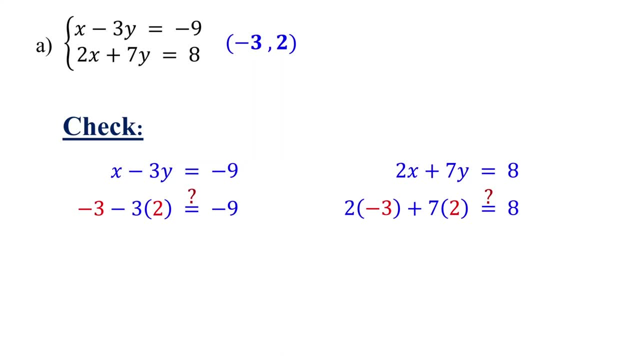 it into both original equations. Substitute negative 3 for x and 2 for y. In the first equation, 3 times 2 is 6.. Negative 3 minus 6 is negative 9.. In the second equation, 2 times negative 3 is negative 6, and 7 times 2 is 14.. 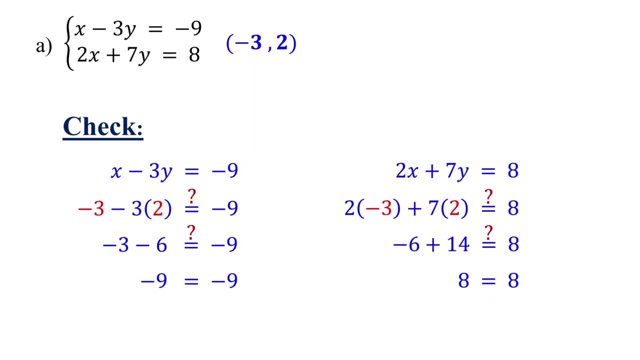 Negative 6 plus 14 is 8.. As you can see, both equations are satisfied, confirming that the ordered pair negative 3 comma 2 is indeed the solution to the system of equations. Now let's try the second example, where the second equation is already solved for y, Since y is already 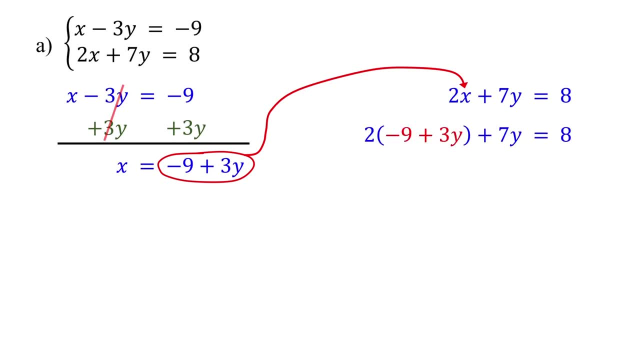 with the equation of x Into the second equation for x. That is why it is called the substitution method. As you can see, we now have an equation with just one variable, and we know how to solve this right. First, let's distribute the two. 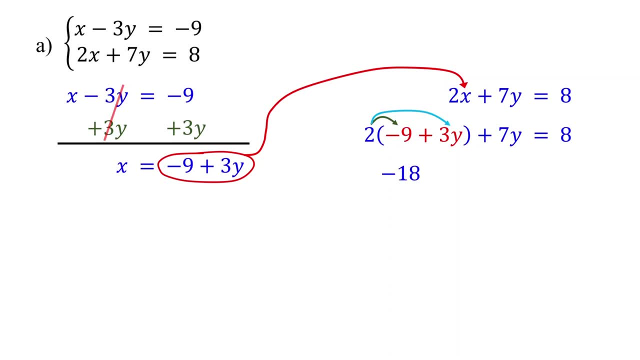 2 times negative. 9 is negative 18.. 2 multiplied by 3y equals 6y. Then combine like terms: 6y plus 7y equals 13y. Then add 18 to both sides of the equation. On the left side the 18s cancel each other out. 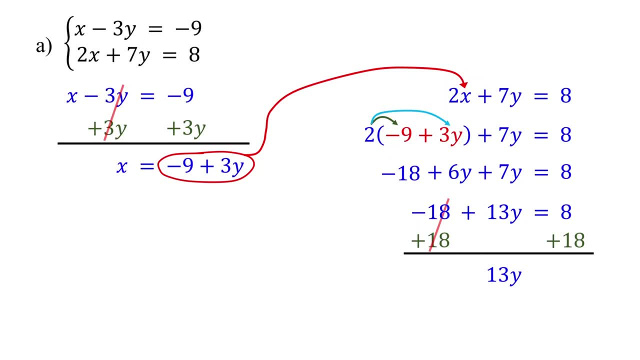 leaving us with 13y On the right side. 8 plus 18 is 26.. Now to isolate y, divide both sides by 13, and you get y equals 2.. Now that we have the value of y, the next step is to find the value of x. 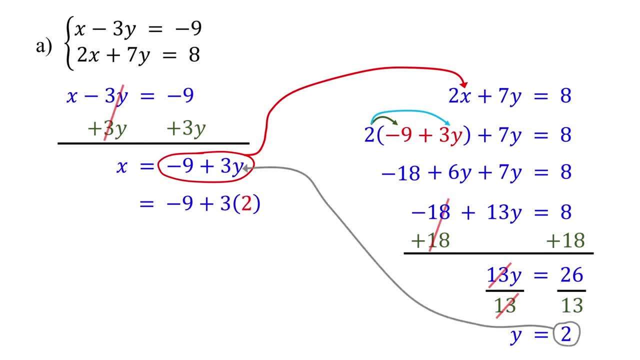 by plugging in 2 for y. in this equation, which is basically the first equation solved for x, 3 times 2 is 6, and negative 9 is negative 9.. 9 plus 6 is equal to negative 3.. Finally, write your solution as an ordered pair. 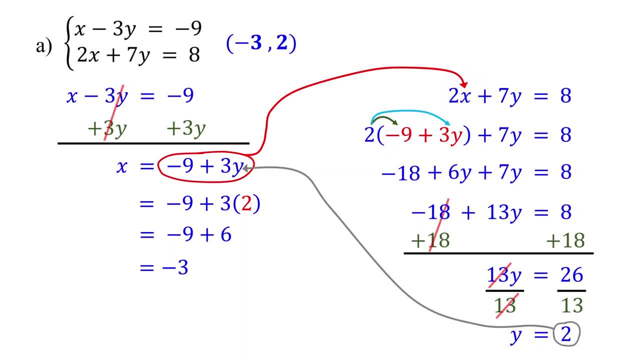 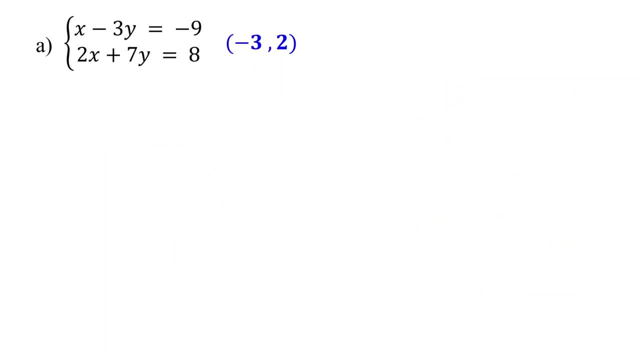 negative 3 comma 2, with x equal to negative 3 and y equal to 2.. If you were to plot the graphs of these two equations, the lines would intersect at a point. negative 3 comma 2.. We can check that the ordered pair is a solution to the system by substituting: 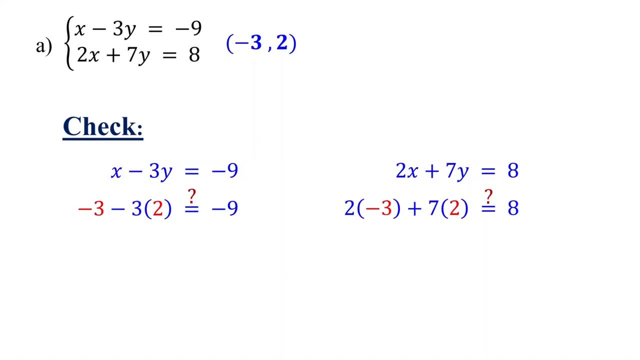 it into both original equations: Substitute negative 3 for x and 2 for y, And this is what we get. In the first equation: 3 times 2 is 6.. Negative 3 minus 6 is negative 9.. In the second equation: 2 times negative. 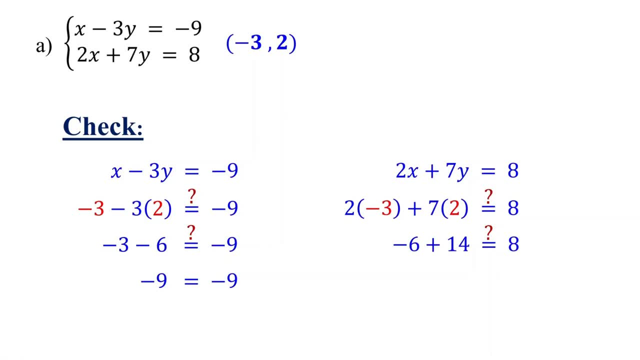 3 is negative 6 and 7 times 2 is 14.. Negative 6 plus 14 is 8.. As you can see, both equations are satisfied, confirming that the ordered pair negative 3 comma 2 is indeed the solution to the system of equations. Now let's try the second example. 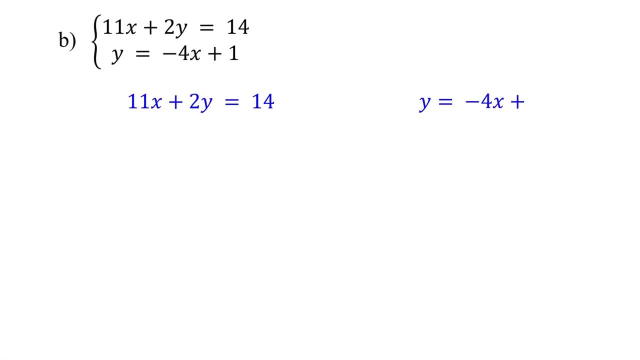 where the second equation is already solved for y. Since y is already isolated in the second equation, we just need to substitute this expression for y into the first equation. Now let's solve this equation for x. First, distribute the two: 2 times negative. 4x is negative 8x. 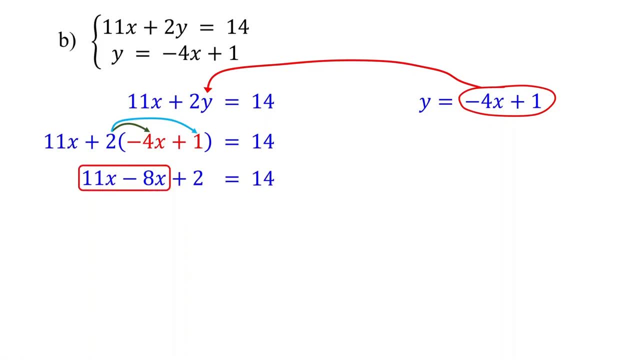 2 times 1 is 2.. Then combine like terms: 11x minus 8x equals 3x. Now subtract 2 from each side of the equation. Cancel these out. 14 minus 2 is 12.. 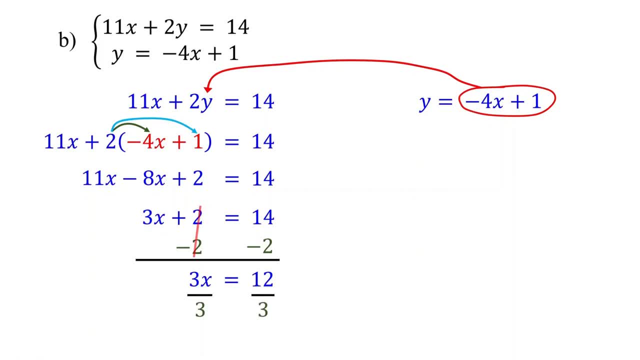 Now divide both sides by 3 to isolate x, And you get x equals 4.. Now that you have the value of x, the next step is to calculate the value of y. You can do that by plugging in 4 for x in the second equation. 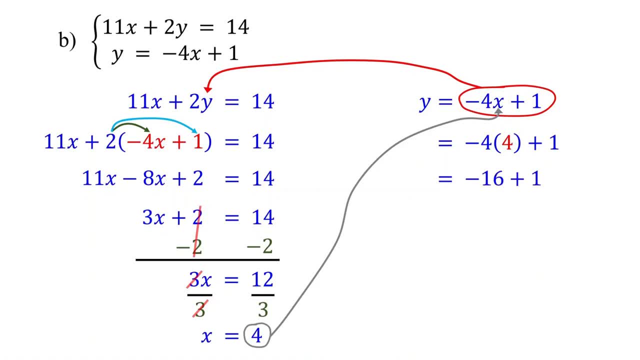 Negative 4 times 4x is negative 4x. Negative 4 times 4 is negative 16.. Negative 16 plus 1 is negative 15.. Therefore, the solution to this system of equations as a coordinate pair is 4 comma negative 15,. 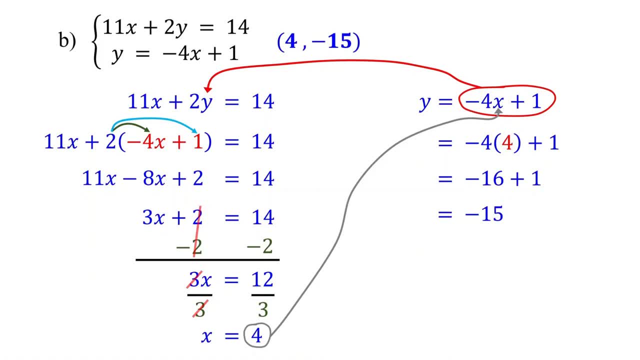 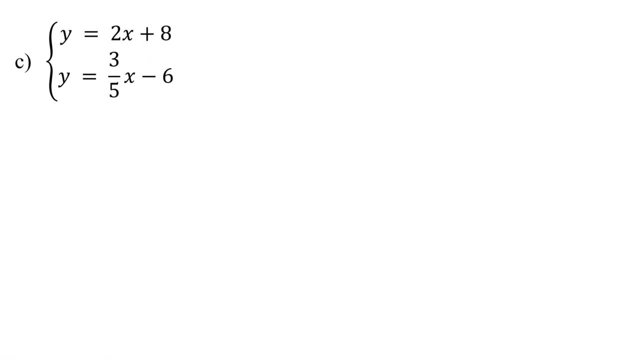 with x equals 4 and y equals negative 15.. In the next example, both equations are solved for y. Please feel free to pause the video and give it a try, Because both equations are already solved for y. you can substitute one into the other. 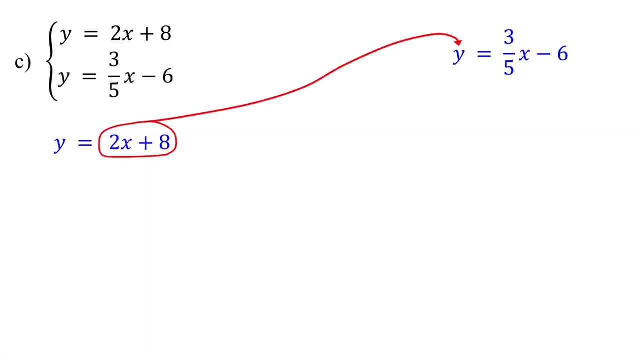 You can substitute this expression for y in the second equation or this expression for y in the first equation. It doesn't matter, You will get the same result in both cases. Let's substitute 2x plus 8 for y in the second equation. 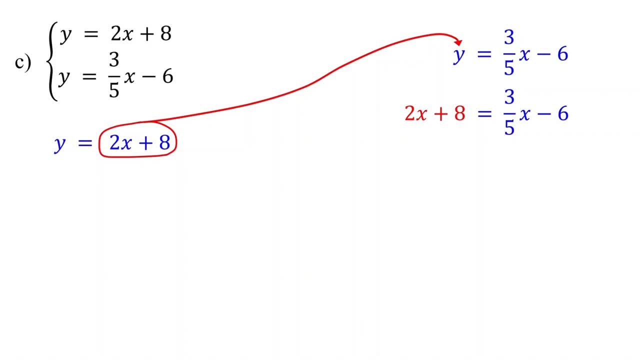 Now, to solve this equation, start by clearing the fraction. To do that, multiply both sides of the equation by 5.. Then distribute the 5 on the left side of the equation. 5 multiplied by 2x equals 3.. 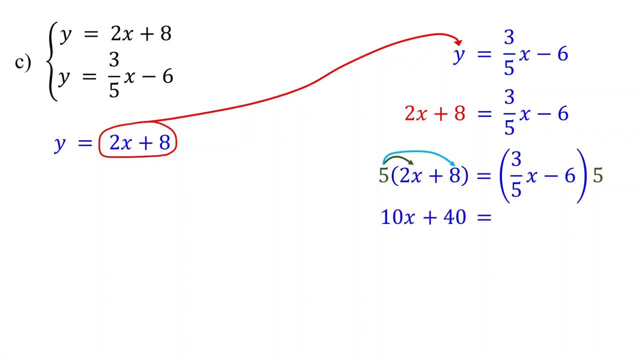 5 multiplied by 2x equals 10x, And 5 multiplied by 8 is 40. Then distribute the 5 on the right side of the equation: 5 multiplied by 3 over 5x equals 3x. 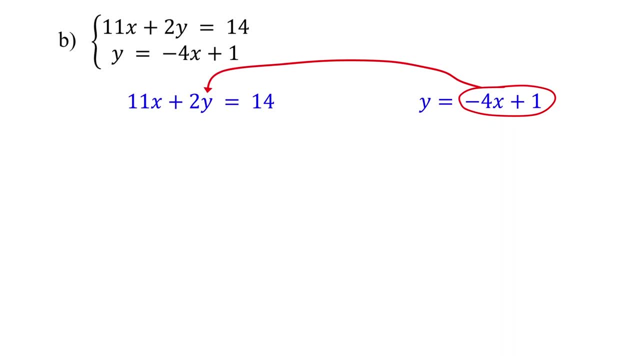 isolated in the second equation. we just need to substitute this expression for y into the first equation. Now let's solve this equation for x. First distribute the two 2 times negative. 4x is negative, 8x 2 times 1 is 2.. Then combine like terms: 11x minus 8x equals. 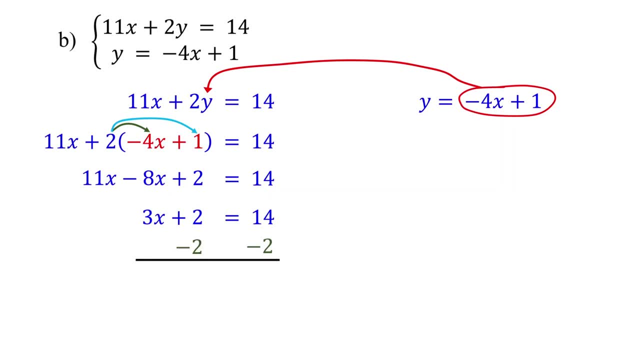 3x. Now subtract 2 from each side of the equation. Cancel these out. 14 minus 2 is 12.. Now divide both sides by 3 to isolate x, And you get x equals 4.. Now that you have, 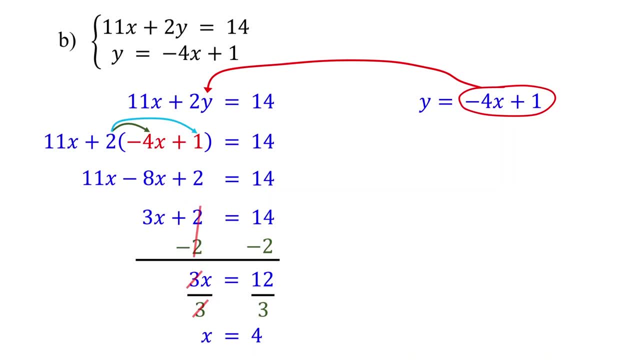 the value of x. the next step is to calculate the value of y. You can do that by plugging in 4 for x in the second equation. Negative 4 times 4 is negative 16.. Negative 4 times 4 is negative 16.. 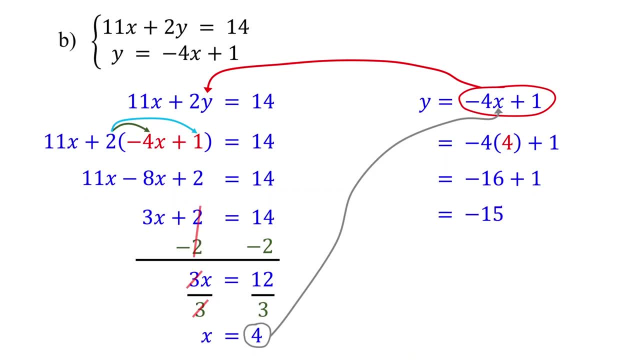 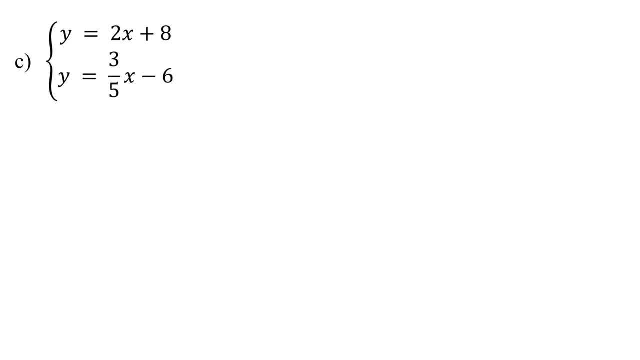 Negative. 16 plus 1 is negative 15.. Therefore, the solution to this system of equations as a coordinate pair is 4 comma negative 15, with x equals 4 and y equals negative 15.. In the next example, both equations are solved for y. Please feel free to pause the video. 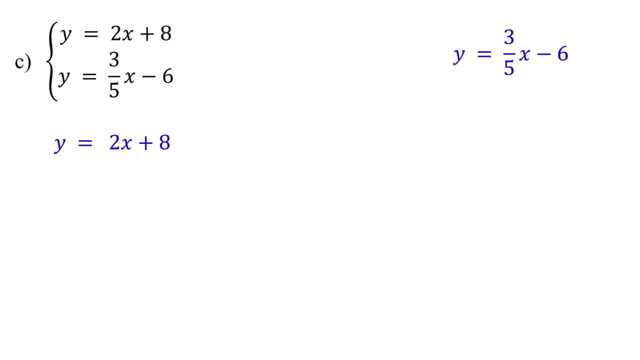 and give it a try, Because both equations are already solved for y. you can substitute one into the other. You can substitute this expression for y in the second equation or this expression for y in the first equation, It doesn't matter, You will get the same result in both cases. 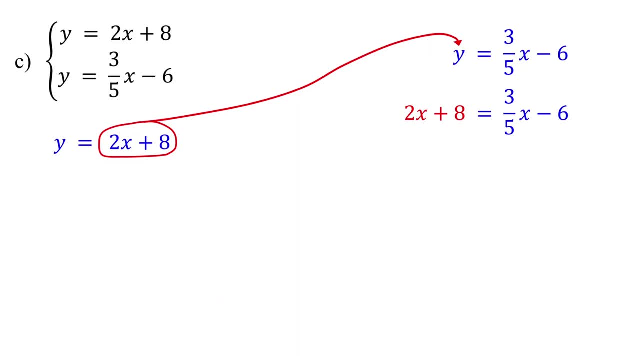 Let's substitute 2x plus 8 for y in the second equation. Now to solve this equation, start by clearing the fraction. To do that, multiply both sides of the equation by 5.. Then distribute the 5 on the left side of the equation: 5 multiplied by 2x equals 10x And 5 times 8. 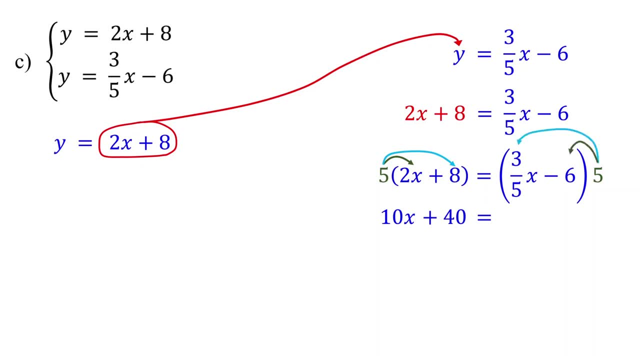 is 40. Then distribute the 5 on the right side of the equation: 5 times 3 over 5x equals 3x right, And 5 times negative 6 is negative 30. Now to get the variable on one side and the. 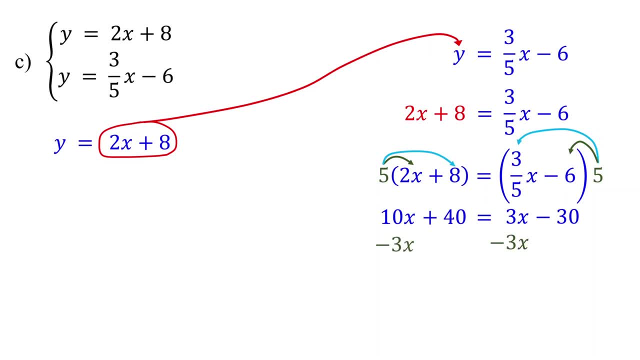 constant. on the other side of the equation, subtract 3x from both sides and, at the same time, subtract 40 from both sides of the equation. On the left-hand side, these cancel out, and 10x minus 3x is 7x. On the right-hand side, cancel these out and negative 30 minus 40 is equal to negative. 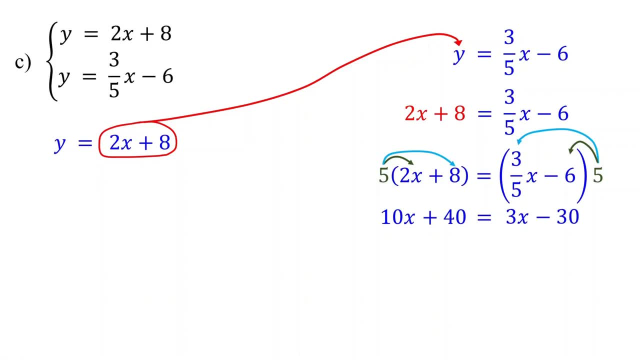 Right, And 5 multiplied by negative 6 is negative 30. Now to get the variable on one side and the constant on the other side of the equation, subtract 3x from both sides and at the same time subtract 40 from both sides of the equation. 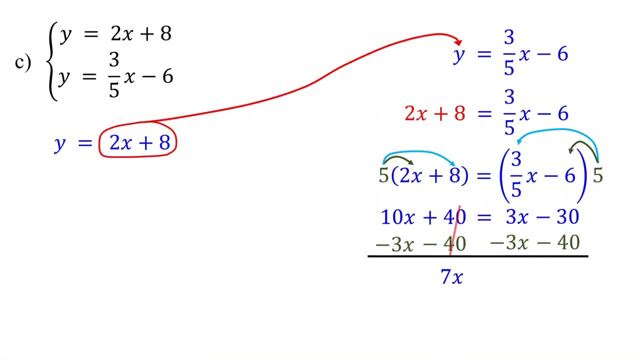 On the left-hand side, these cancel out, and 10x minus 3x is 7x. On the right-hand side, cancel these out and negative 30 minus 40 is equal to negative 70.. Now to isolate x, divide both sides by 7.. 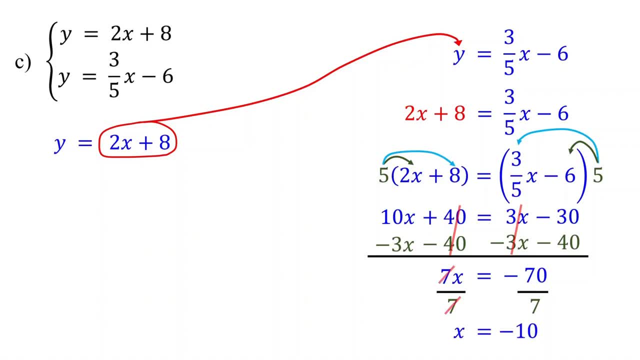 And you get x equals negative 10.. Next, plug in this value of x into the first equation to find the value of y. 2 times negative 10 is negative 20.. Negative 20 plus 8 is equal to negative 12.. 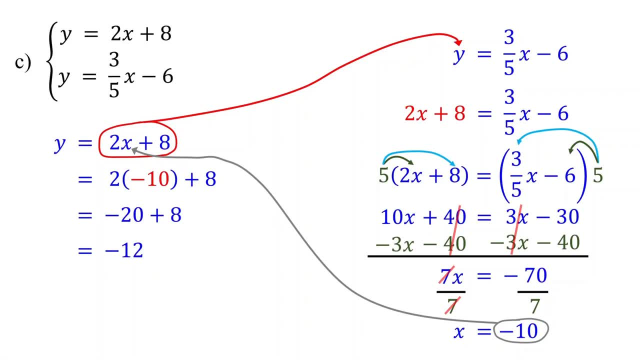 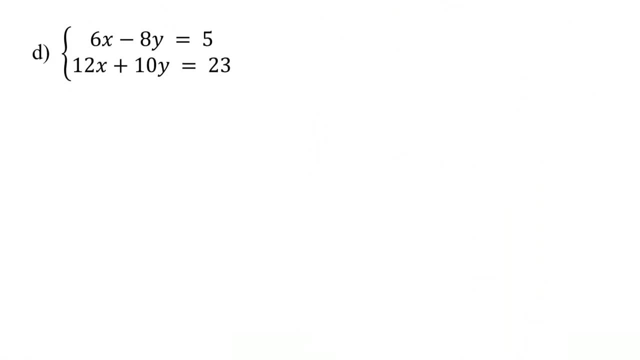 Therefore the solution to this example is negative, 12 comma, negative, 10.. The next example is a bit challenging. In both equations, neither variable is isolated and neither coefficient is equal to 1.. In systems of equations like these, the elimination method is often the most straightforward approach for solving them. 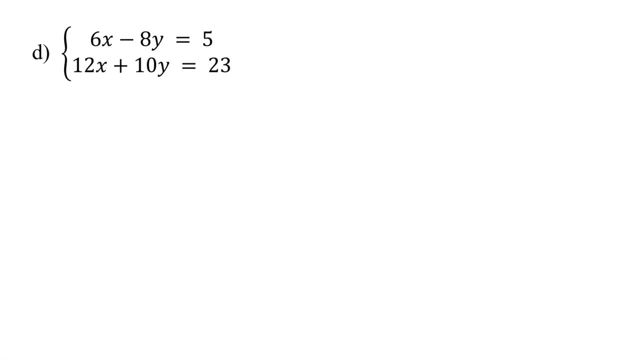 However, sometimes you may be given a problem like this and asked to use the substitution method. You will follow the same steps as in the previous examples. The first step is to isolate either x or y in one of the equations. Let's isolate x in the first equation. 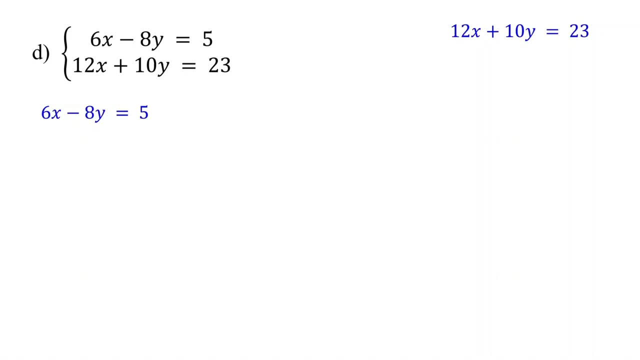 I will explain shortly why I chose the first equation and decided to isolate x. First, add 8y to both sides of the equation. These cancel out and you get 6x equals 5 plus 8y. Now divide both sides by 6.. 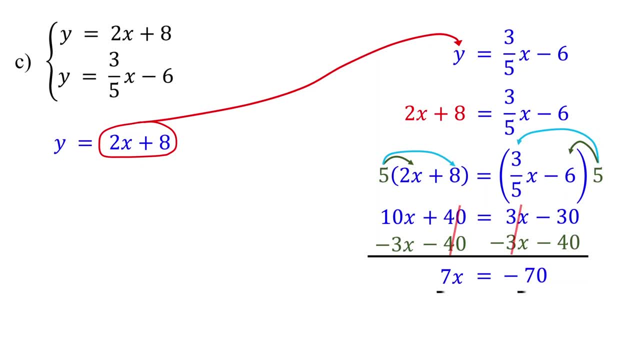 70. Now to isolate x, divide both sides by 7 and you get x equals negative 10.. Next, plug in this value of x into the first equation to find the value of y. 2 times negative. 10 is negative 20.. 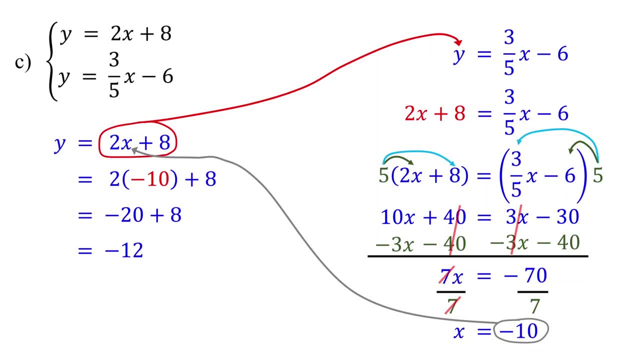 Negative 20 plus 8 is equal to negative 12.. Therefore the solution to this example is negative 12 comma, negative 10.. The next example is a bit challenging. In both equations, neither variable is isolated and neither coefficient is equal to 1.. 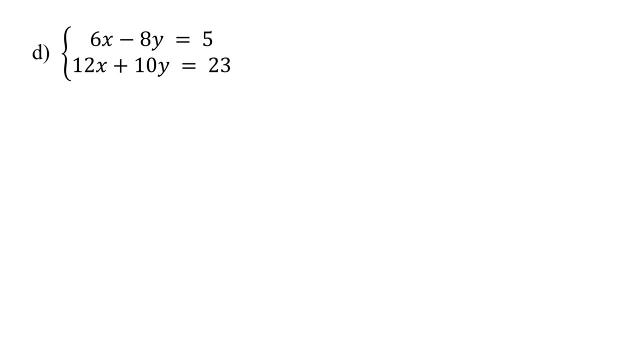 In systems of equations like these, the elimination method is often the most straightforward approach for solving them. However, sometimes you may be given a problem like this and asked to use the substitution method. We will follow the same steps as in the previous examples. 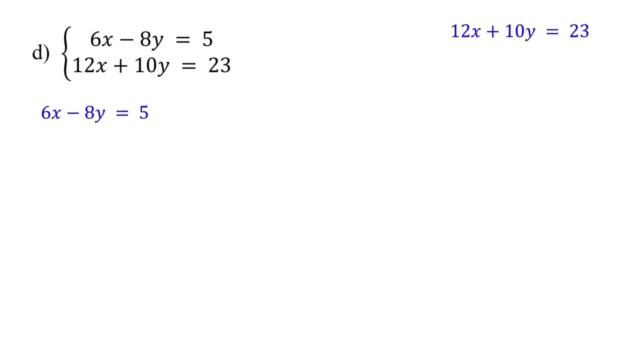 The first step is to isolate either x or y in one of the equations. Let's isolate x in the first equation. I will explain shortly why I chose the first equation and decided to isolate x First. add 8y to both sides of the equation. These cancel out and you get 6x equals 5 plus 8y. 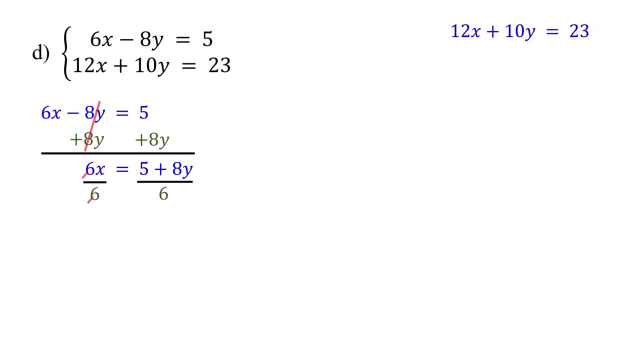 Now divide both sides by 6. So you have x equals 5 plus 8y over 6.. Now divide both sides by 6. So you have x equals 5 plus 8y over 6.. Now that we have x by itself in the first equation, the next step is to substitute this: 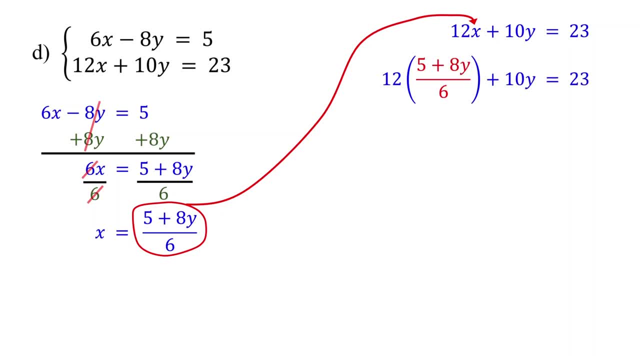 expression for x into the second equation On the left side of the equation. simplify by dividing both 12 and 6 by 6, resulting in 2.. This simplifies the equation to 2 times 5 plus 8y plus 10y equals. 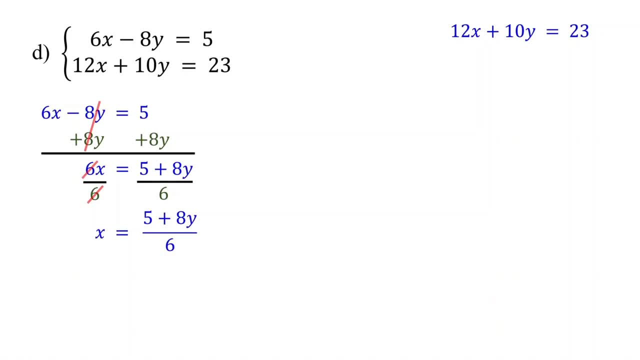 So you have: x equals 5 plus 8y over 6.. Now that we have x by itself in the first equation, the next step is to substitute this expression for x into the second equation. On the left side of the equation, simplify by dividing both 12 and 6 by 6, resulting in 2.. 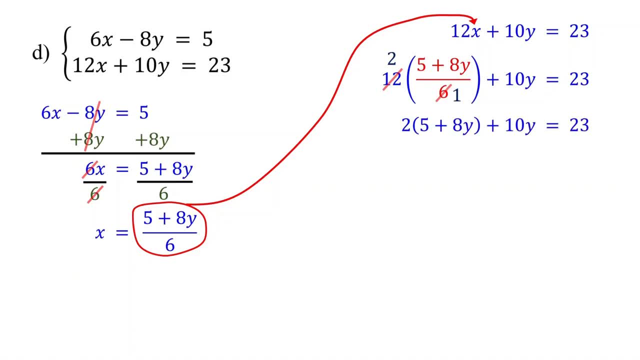 This simplifies the equation to 2 times 5 plus 8y plus 10y equals 23.. Notice that there are no fractions in this equation. Initially I observed that isolating x in the first equation would introduce a fraction with 6 in the denominator of the expression. 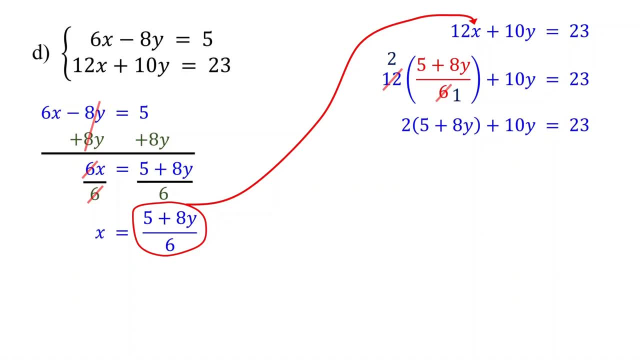 However, I noticed that when substituting this expression for x into the second equation, we can eliminate the fraction because 12 is divisible by 6, making the expression simpler to work with. That's why I chose the first equation and decided to isolate x. 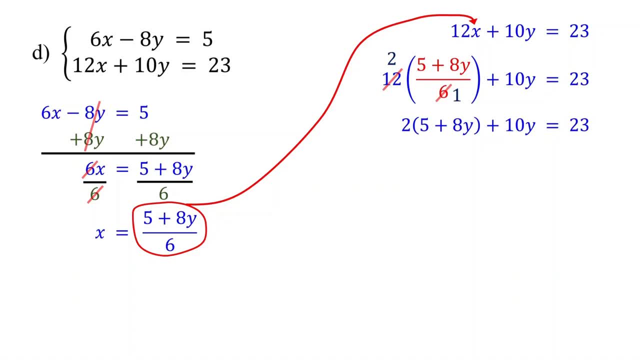 If we had chosen to isolate y in the first equation, we would still have fractions at this step. This is because isolating y results in an 8 in the denominator of the expression and when we substitute it for y in the second equation. 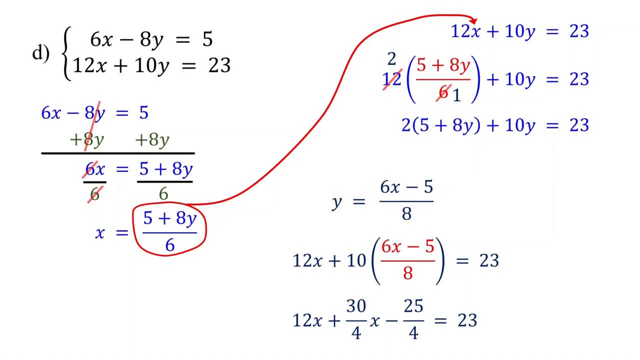 we cannot eliminate the fraction, as 10 is not divisible by 8. This would complicate the calculations and require additional steps. The same applies if we had chosen the second equation and isolated either x or y: We would still have fractions, making the calculations more challenging. 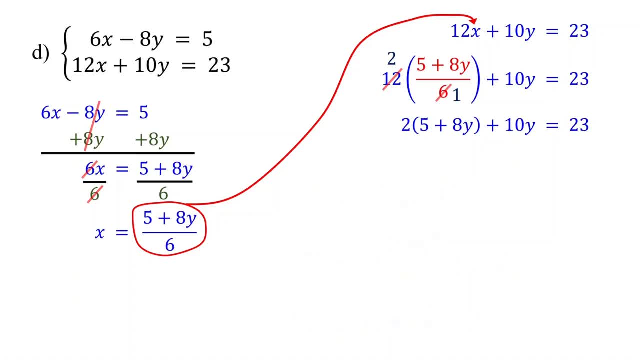 So, whenever possible, pick an equation and a variable that make the work easier. Having said this, now let's go ahead and distribute the two: 2 times 5 is 10, and 2 times 8y is 16y. 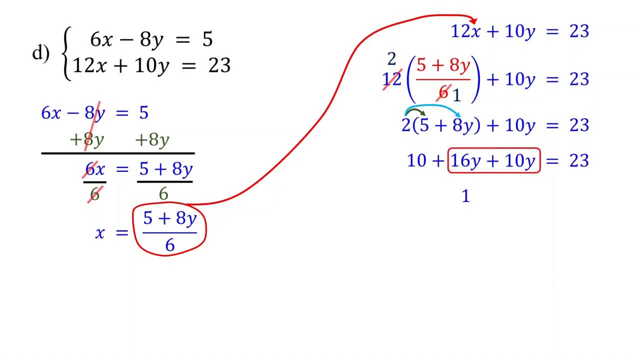 Then combine like terms. Adding this, we get 26y right Now. subtract 10 from each side of the equation. Cancel these. 23 minus 10 is 13.. To isolate y divide both sides by 26.. 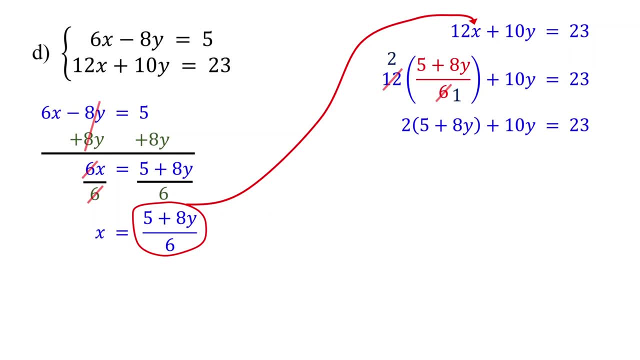 23. Notice that there are no fractions in this equation. Initially I observed that isolating x in the first equation would introduce 2 times 5 plus 8y. Now divide both sides by 6 and 6 by 6.. 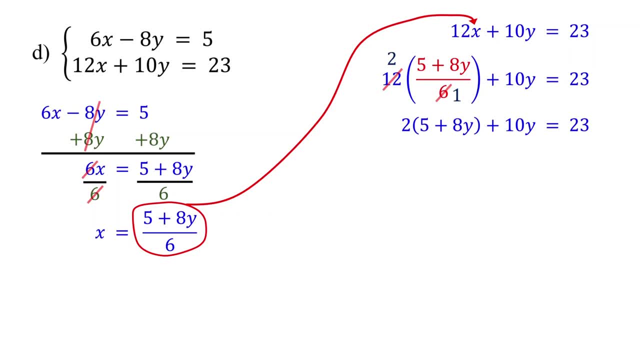 Finally, the slightly smaller fraction which is coming with x equals 5 plus 8y would introduce a fraction with 6 in the denominator of the expression. However, I noticed that when substituting this expression for x into the second equation, we can eliminate the fraction because 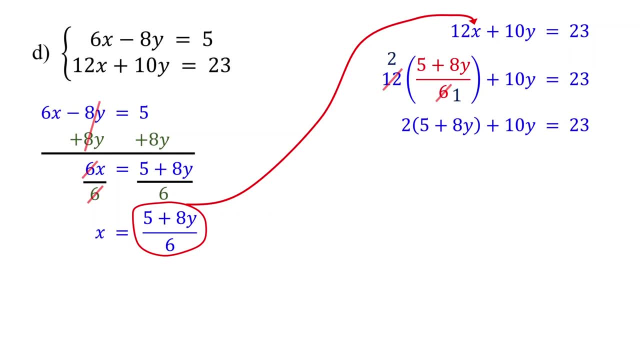 12 is divisible by 6, making the expression simpler to work with. That's why I chose the first equation and decided to isolate x. If we had chosen to isolate y in the first equation, we would still have fractions at this step. This is because isolating y results. 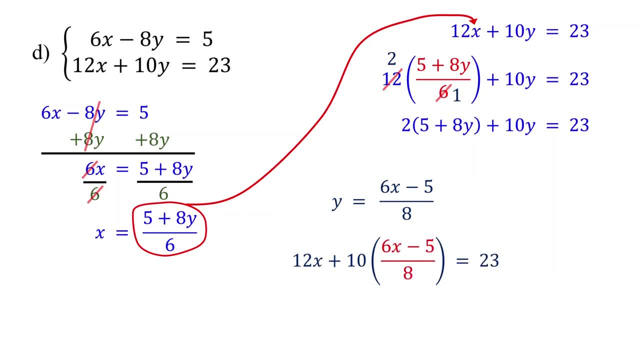 an 8 in the denominator of the expression and when we substitute it for y in the second equation, we cannot eliminate the fraction, as 10 is not divisible by 8.. This would complicate the calculations and require additional steps. The same applies if we had chosen the second equation and isolated either x or y. 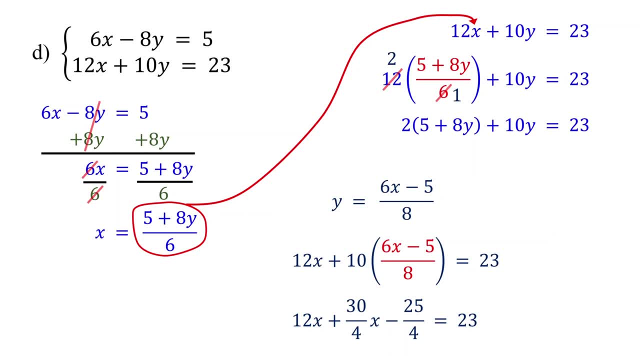 We would still have fractions, making the calculations more challenging. So, whenever possible, pick an equation and a variable that make the work easier. Having said this, now let's go ahead and distribute the two. Two times five is ten, and two times eight, y is sixteen, y. 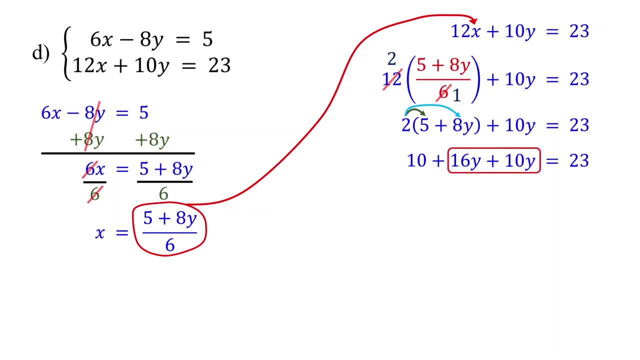 Then combine like terms. Adding this, we get twenty-six y. right Now. subtract ten from each side of the equation. Cancel these. Twenty-three minus ten is thirteen. To isolate y divide both sides by twenty-six. You can simplify thirteen over twenty-six to 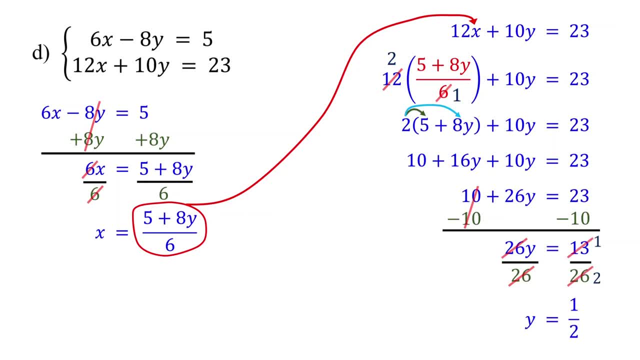 one-half, So y is equal to one-half. Next, find the value of x by plugging in one-half for y in this equation, Eight times one-half is four, And five plus four is nine. If we divide both nine and six by three, we can simplify it to three-halves. 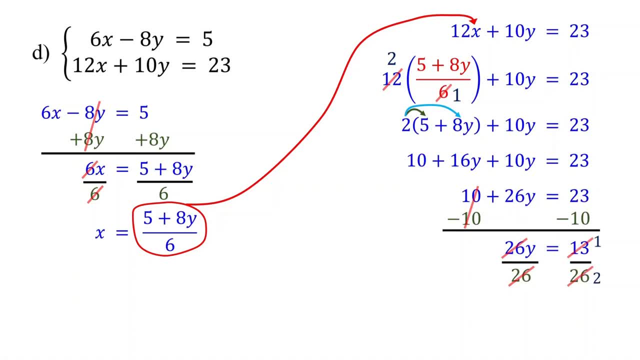 You can simplify 13 over 26 to 1 half, So y is equal to 1 half. Next, find the value of x by plugging in 1 half for y. in this equation, 8 times 1 half is 4.. 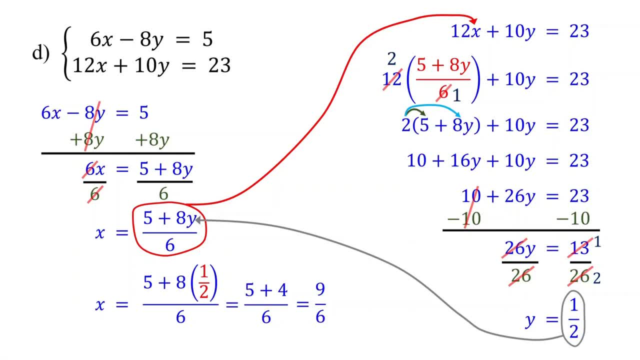 And 5 plus 4 is 9.. If we divide both 9 and 6 by 3, we can simplify it to 3 halves. Therefore, the solution to this system of equations is: 3 halves, comma, 1 half. The examples we have solved so far have exactly one solution. 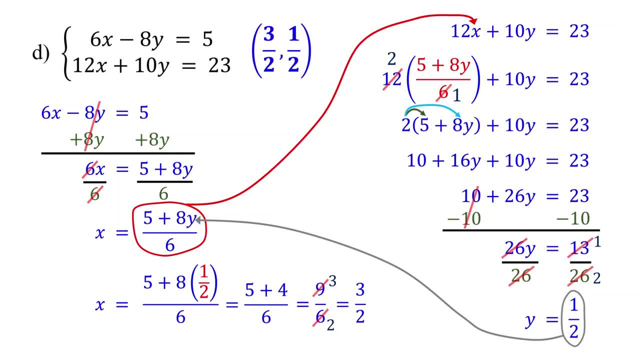 Therefore, the solution to this system of equations is three-halves comma one-half. The examples we have solved so far have exactly one solution. In the next two examples we will use the same solution. In the next two examples we will see two special cases where the system of equations 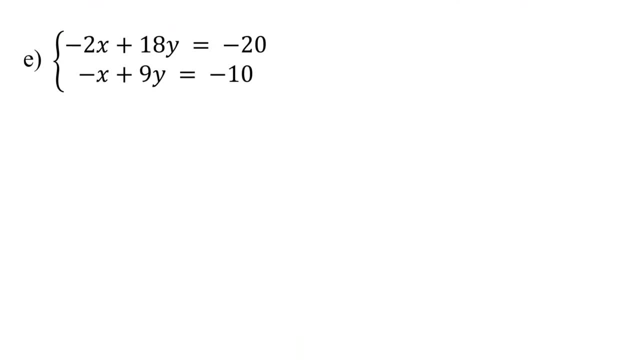 has infinitely many solutions and no solution. If you have any questions, please feel free to leave them in the comments below. Since the coefficient of the x variable in the second equation is negative one, it is easier to solve for x in the second equation. 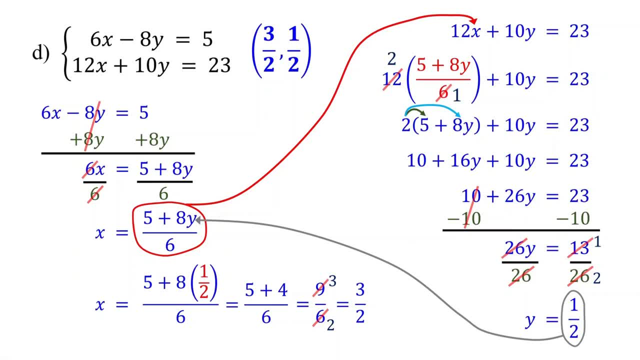 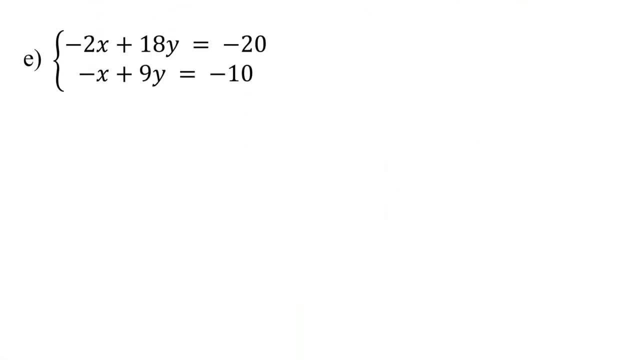 In the next two examples we will see two special cases where the system of equations has infinitely many solutions and no solution. If you have any questions, please feel free to leave them in the comments below. Since the coefficient of the x variable in the second equation is negative 1,, it is easier to solve for x in the second equation. 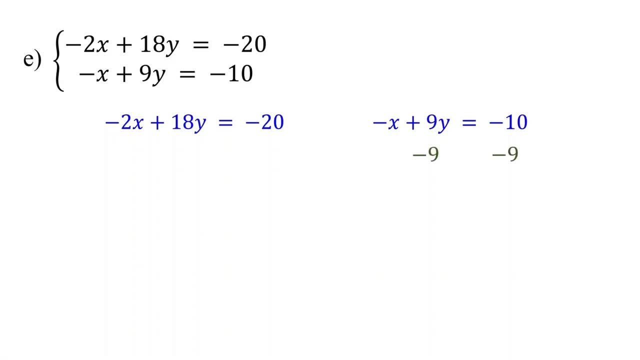 So let's do that. First, subtract 9y from each side of the equation. Cancel these and you get negative x equals negative 10 minus 9y. Now, to get rid of the negative sign in front of x, multiply both sides of the equation by negative 1.. 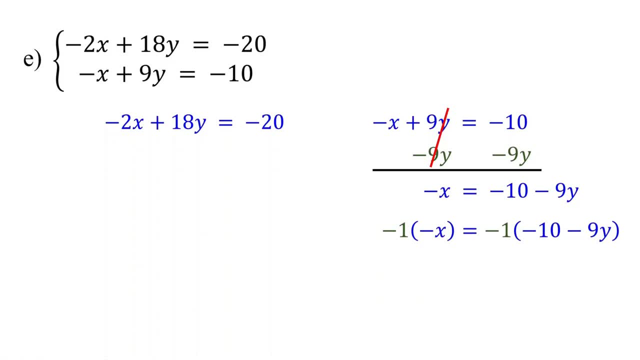 On the left side: negative 1 times negative. x is positive, x. On the right side. distribute negative: 1. Negative 1 times negative. 10 is positive 10. Negative 1 times negative: 9y is positive 9y. 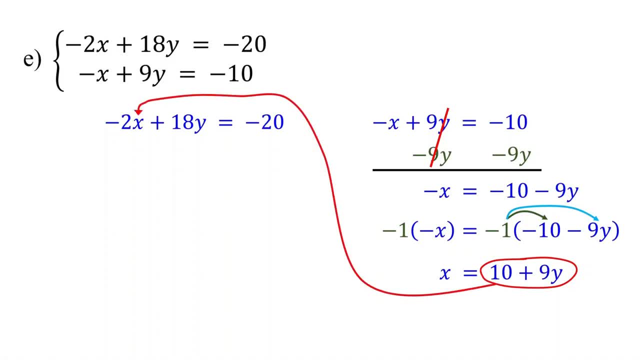 Next substitute this expression for x into the first equation. Now distribute negative: 2.. Negative 2 times 10 is negative 20.. Negative 2 times 9y equals negative 18y. Then combine like terms. This adds up to 0. 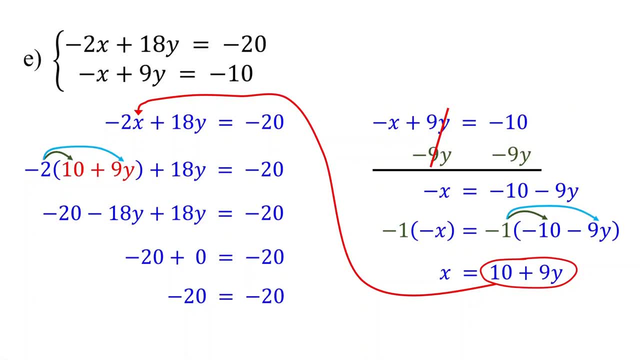 So we have negative 20 equals negative 20, which is indeed true. This indicates that the system of equations has infinitely many solutions, Which means there are an infinite number of ordered pairs that satisfy both equations simultaneously. If you were to plot the graphs of these two equations, the lines would coincide perfectly, indicating that any point on the lines satisfies both equations. 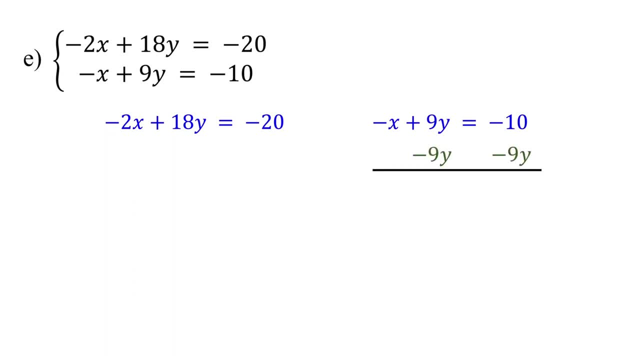 So let's do that. First, subtract nine y from each side of the equation. Cancel these and you get negative x equals negative ten minus nine y. Now, to get rid of the negative sign in front of x, multiply both sides of the equation. 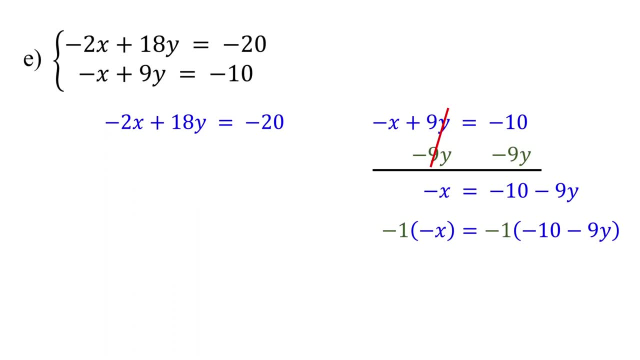 by negative one On the left side. negative one times negative. x is positive x On the right side. distribute negative one, Negative one times negative. ten is positive ten Negative one times negative. nine y is positive nine y. Next. substitute this expression for x into the first equation. 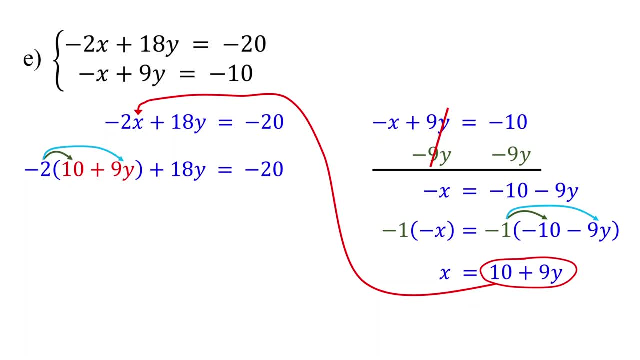 Now distribute negative x. Now distribute negative x. negative two: Negative two times ten is negative twenty. Negative two times nine: y equals negative eighteen y. Then combine like terms. This adds up to zero. So we have negative twenty equals negative twenty, which is indeed true. 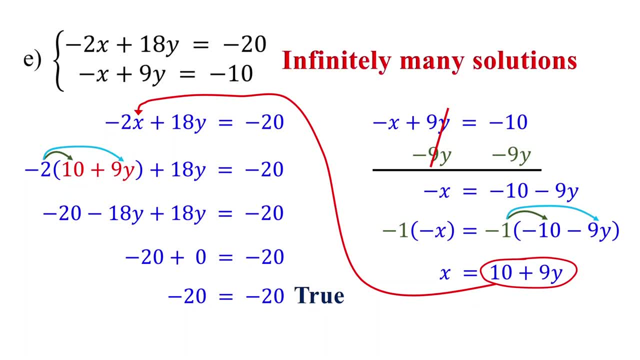 This indicates that the system of equations has infinitely many solutions, which means there are an infinite number of ordered pairs that satisfy both equations simultaneously. If you were to plot the graphs of these two equations, the lines would coincide perfectly, indicating that any point on the lines satisfies both equations. 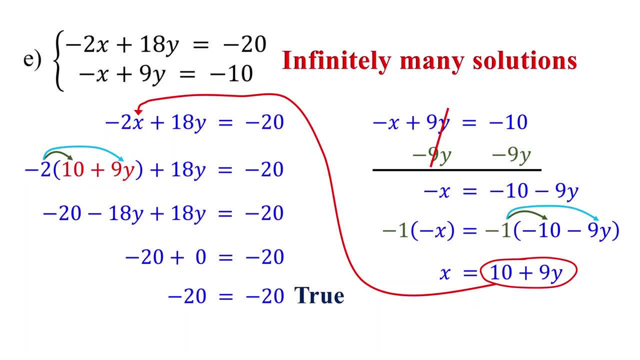 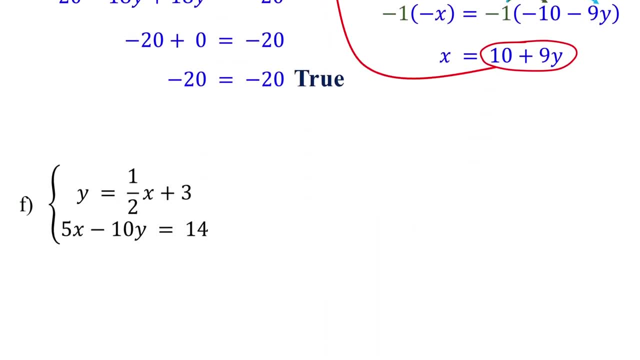 So when you solve a system of equations and end up with a number equal to itself, as in this example, the answer is infinitely many solutions. Finally, let's consider the case where the system of equations has no solution. As you can see, the first equation is already solved, for y. 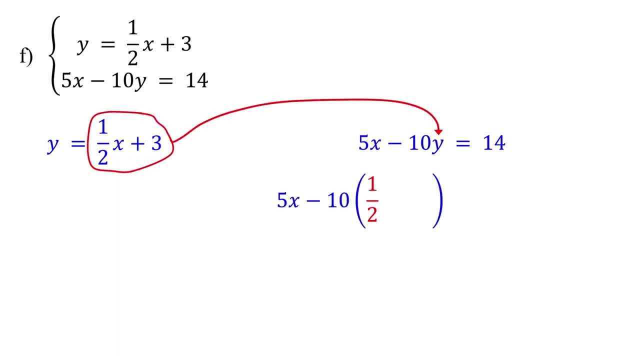 so you can substitute this expression directly into the second equation for y. Now to solve this equation, start by distributing negative 10.. Negative 10 times 1 over 2x equals negative 5x. Negative 10 times 3 is negative 30.. 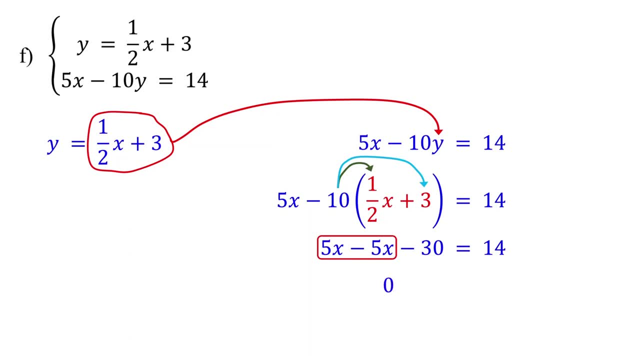 Then combine like terms. Subtracting this give us 0, so we have negative. 30 equals 14, which is false. This indicates that the system of equations has no solution. It means that there is no ordered pair that satisfies both equations simultaneously. 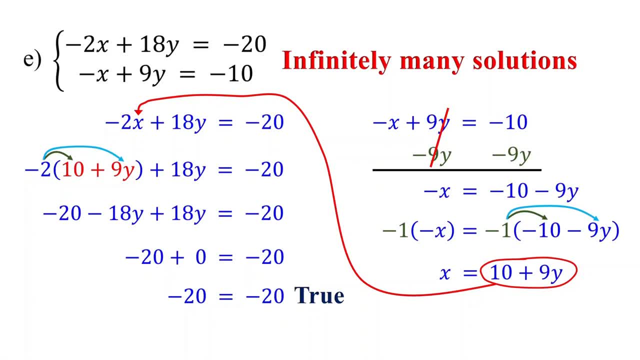 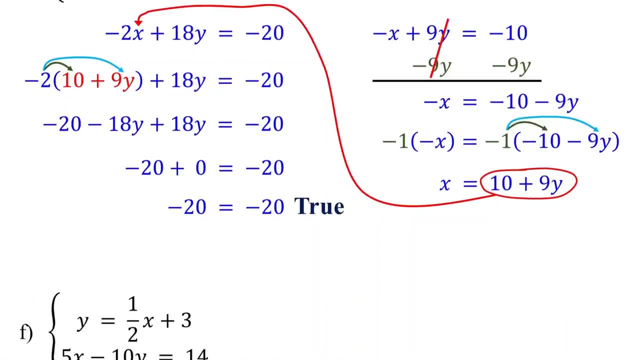 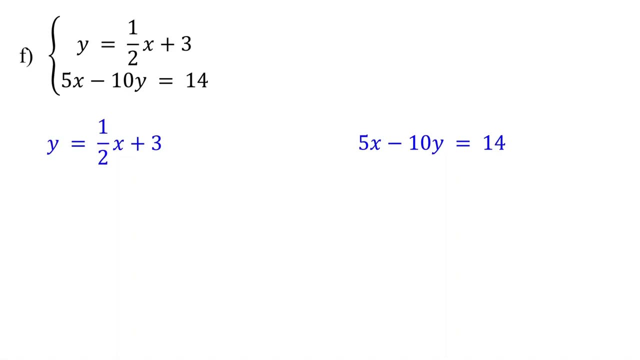 So when you solve a system of equations and end up with a number equal to itself, as in this example, the answer is infinitely many solutions. Finally, let's consider the case where the system of equations has no solutions. As you can see, the first equation is already solved for y, so you can substitute this expression directly into the second equation, for y. 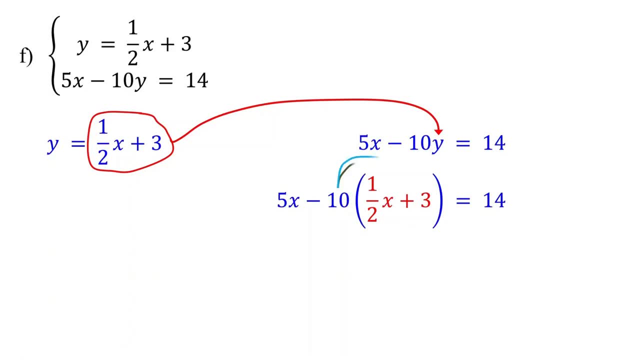 Now to solve this equation, start by distributing negative 10.. Negative 10 times 1 over 2x equals negative 5x. Negative 10 times 3 is negative 30.. Then combine like terms. Subtracting this give us 0.. 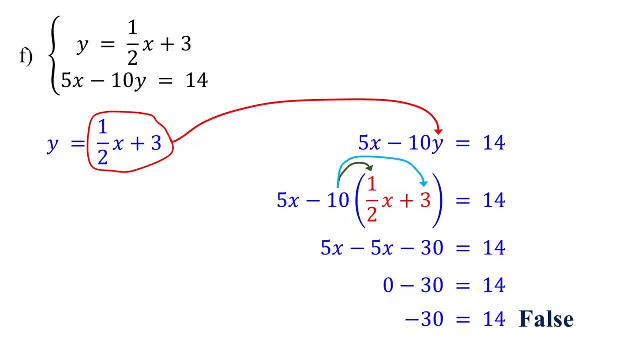 So we have negative 30 equals 14,, which is false. This indicates that the system of equations has no solution. It means that there is no ordered pair that satisfies both equations simultaneously. If you plot the graphs of these two equations, you will notice that the lines do not intersect. 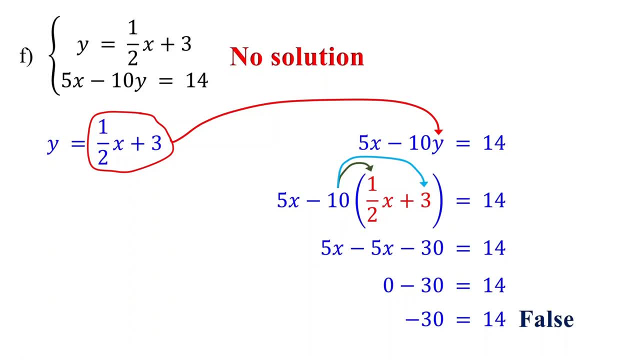 They are parallel lines. So when you solve a system of equations and end up with numbers that are not equal to each other, as in this example, the answer is no solution. Thanks for watching. If you found this video helpful, please give it a thumbs up and subscribe. 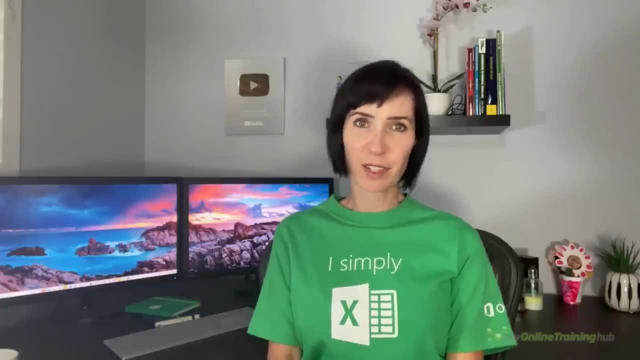 In this video, I'm going to teach you some different ways to visualize year-on-year data, and you'll see that the message conveyed depends on the chart you choose. Line charts are great at displaying data over time, and we can start the vertical axis above zero to accentuate changes. 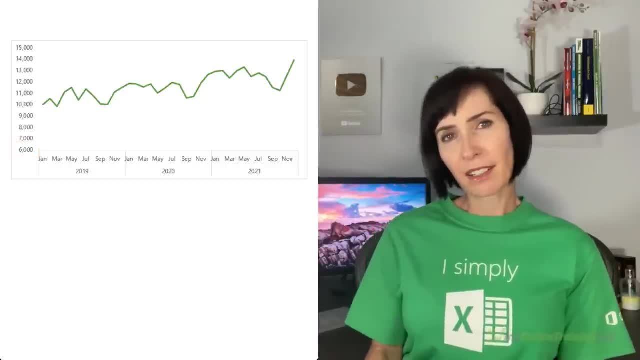 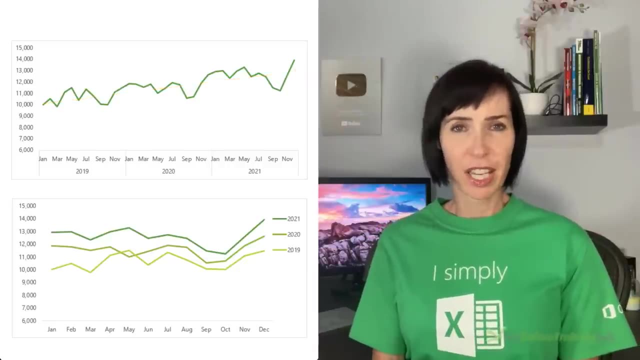 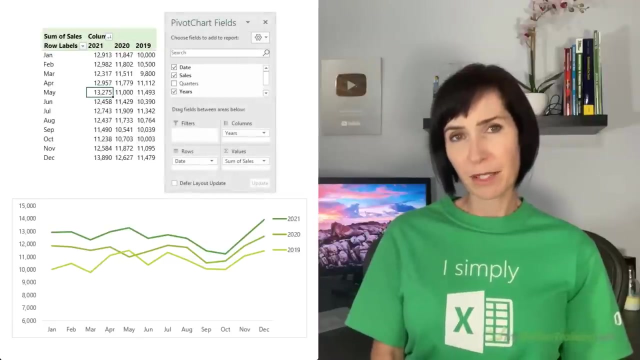 in the data. For example, in this chart, we can see at a glance that the trend is upward, whereas this chart shows the same data with a separate data series for each year, which more clearly illustrates seasonality in the data. The key to generating a chart like this is to format your data with 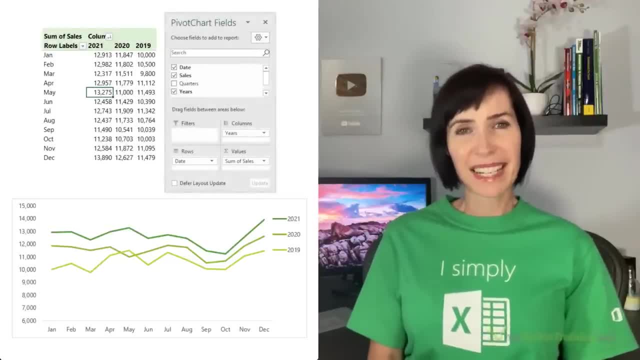 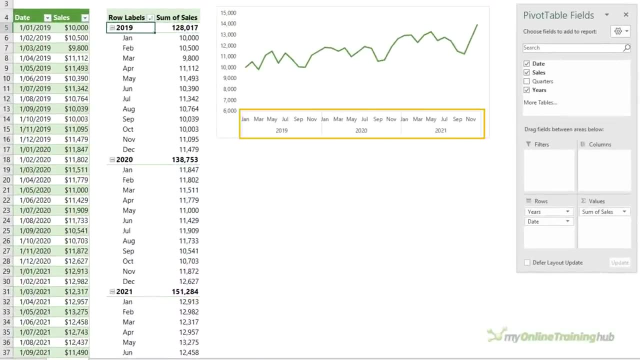 the years in the columns and the months in the rows. Let's take a look. The most common line chart simply shows the data over a continuous timeline and this illustrates the trend really well. Notice the chart. source data has the years and months in the row. labels of the pivot table. 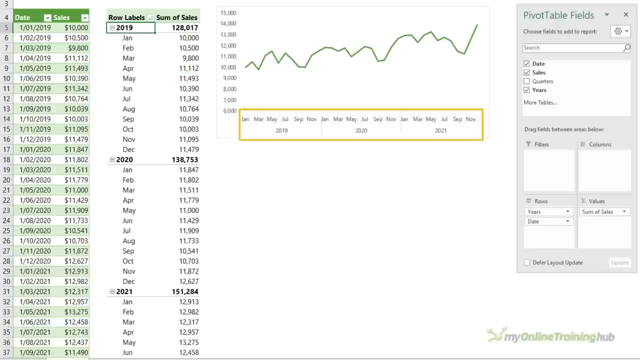 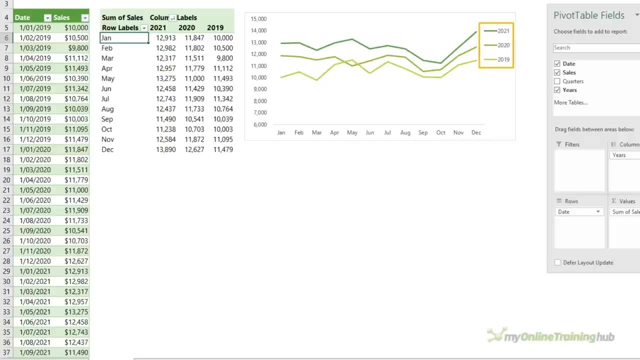 and this results in a continuous date axis with nested year and month labels, Whereas this line chart has a separate series for each year, allowing you to more easily see seasonality in the data, and we achieve this by putting the years in separate columns and the months in the row labels. If you're able to, it's a good idea to align the legend to the lines in the 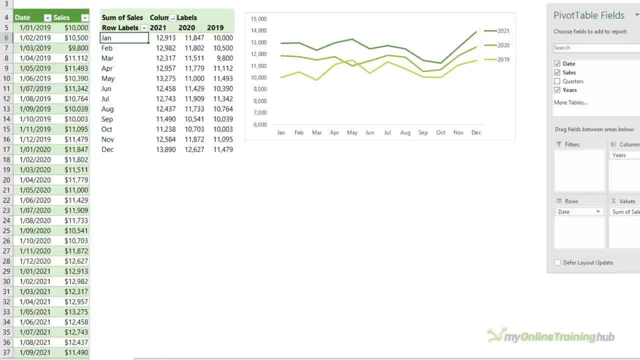 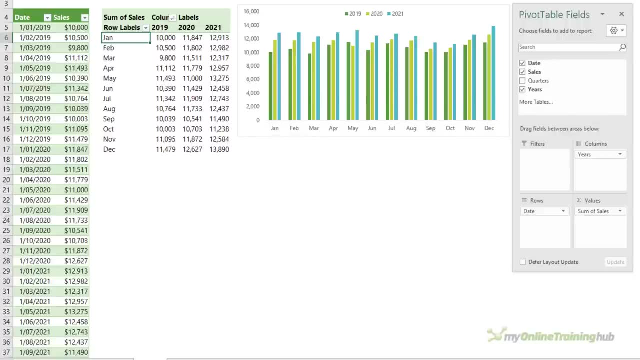 chart. this just makes it quicker and easier for your audience. Column charts are another common way to display year-on-year data. however, notice that even with the change in the color scheme for year-on-year data, it's not as easy to see the trend in the data or compare one year to the other.